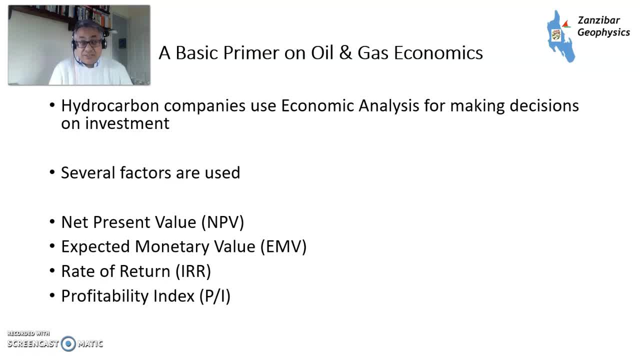 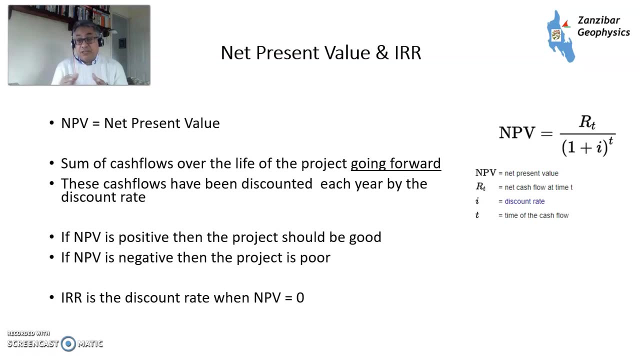 into account. I did a video earlier on using Bayesian theory in making economic decisions. Please have a look on that- and that explains EMV a little bit better. So what is net present value? So it's the sum of cash flows over the life of project going forwards from today. 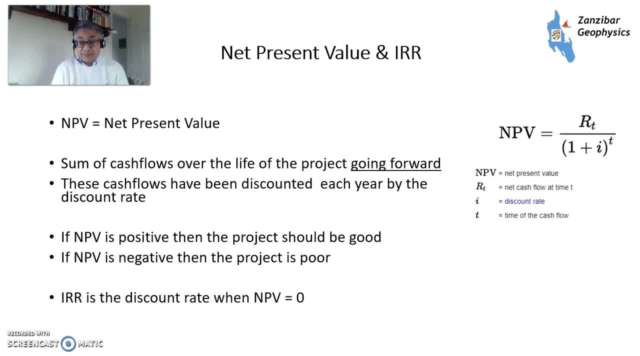 So we ignore what is spent before, so some cost fallacy doesn't happen looking forward, and we discount these cash flows each year by the discount rate because of the time value of money. If the NPV is positive, then the project should be good. If the NPV is negative, then the project to be poor. It's not quite as simple as that, because 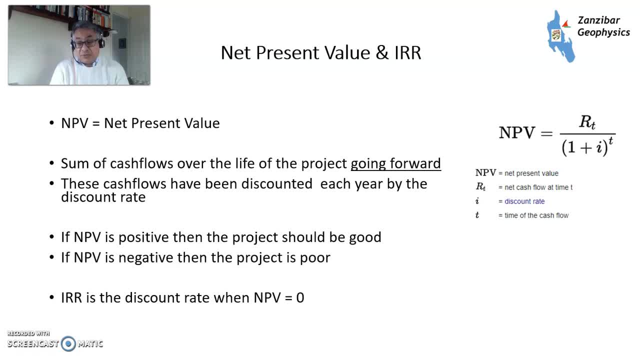 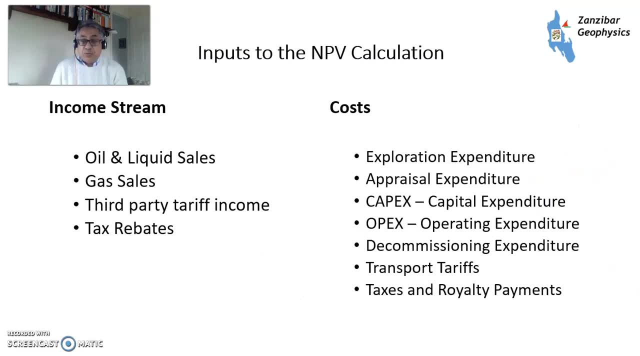 companies have hurdles and the internal rate of return is the discount rate, with the NPV equals 0. And here's the 4.5.. The final formula for those who are formal minded. so what do we have as inputs? We've got our income streams, so that's: oil and liquid sales, gas sales, third party tariff income. 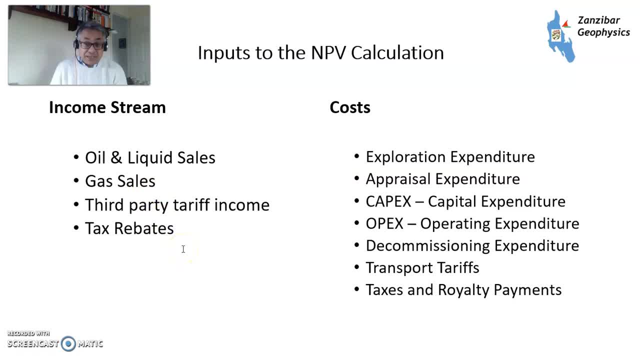 if we're using a facility to host other facilities and any tax rebates that we may have. Particularly, we can offset expiration etc against tax And our costs are the expiration expenditure, appraisal expenditure, CAPEX, which is capital expenditure involved in the業. 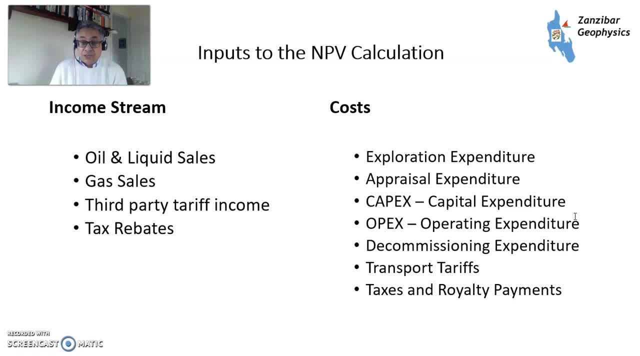 and setting up the field, so that's drilling wells, installing facilities, etc. operating expenditure, which is the daily uh cost of actually producing. so that's both fixed opex and variable opex which is related to production. decommissioning expenditure far forward into the future where we clean up and remediate the site. any transport tariffs- so if we have to pay tariffs, 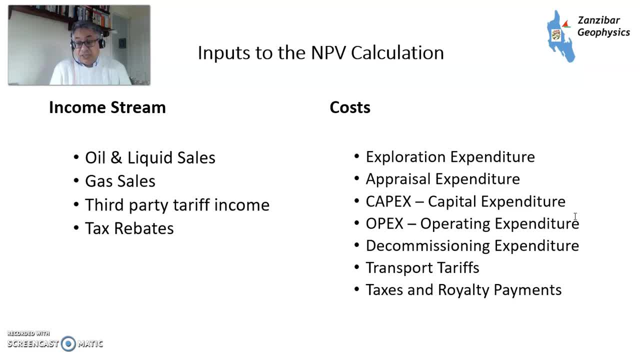 to a third party for processing our hydrocarbons. we pay those, and also taxes and royalty payments, depending on the different type of fiscal regime that the country that we operate has. i've got a video on that as well. so a little bit about hurdle rates now. 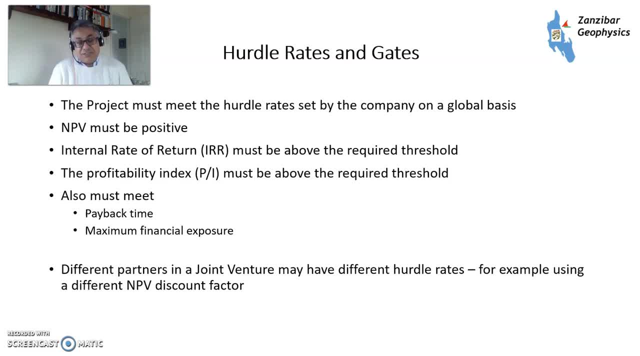 obviously uh, which i'll just say. it's got an mpv of positive. therefore we go ahead. different companies look at different things. now, obviously, the mpv has to be positive. internal rate of return might need to be above a certain threshold. generally, that's to do with: 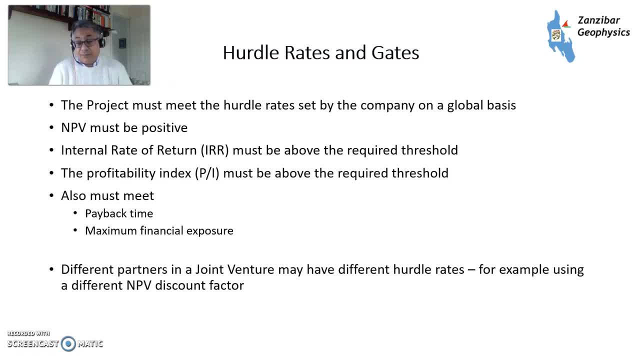 the weighted cost of capital of a company. i'll come to to why that might be important, etc. then there's a profitability index: p over. i needs to be above required threshold. uh, you must also have a little look at payback time and maximum financial exposure. so if you're down 3 billion at the 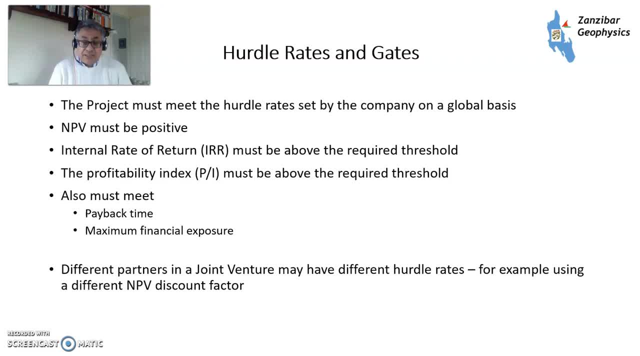 at the peak rate. that might be a little bit hard to do and different partners within a joint venture may have different hurdle rates and they may use a different mpv discount factor, which can be a bit of a problem in some joint ventures. price decks- now a price deck- is a common set of assumptions. 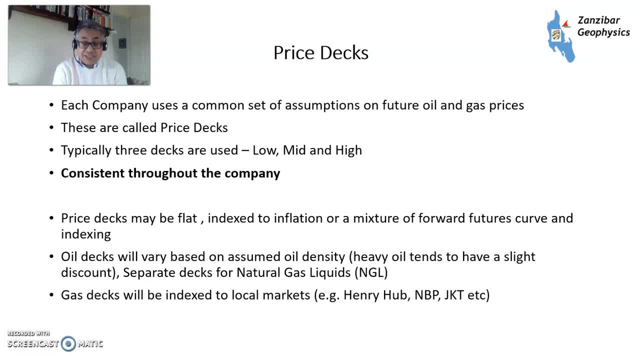 used throughout an organization for future oil and gas companies and generally people would tend to use three price decks. there's would be a low and near than a high, and that would vary along amongst companies. it would vary also through time, so each year you may use a different price deck, depending 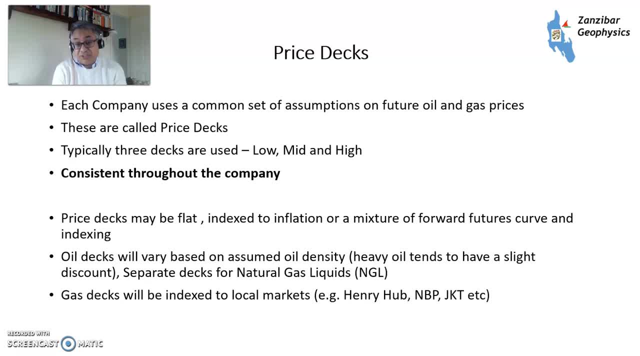 on what, uh, the market fundamentals part of the economics department thinks is going to be the future. price decks could be flat, so let's say, for sake of argument, fifty dollars flat to eternity. or it could be indexed to inflation. it could be a major forward curve. so that's uh from the futures. 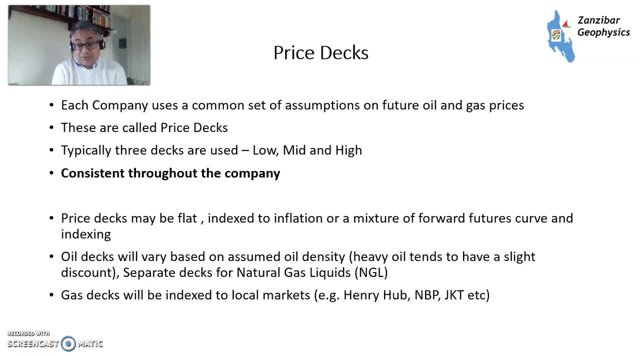 market indexing, etc. you would have variations within the oil price deck depending on the density of the oil. heavy oil tends to have a slight discount. there will be separate decks for natural gas liquids, which again have different, different uh values, and there could be gas decks index larger local markets such as Henry Hub, MBP, JKT LNG prices. I have a video when a BOE is not a BOE. which explains the difference. up to that at prixagifanaianacomau KCM article. so be sure to get orders for more confirming the meidäninals articles. So at prixagifinaianacomau, if you're interested in normal, put también lo que dirán y comparten en el Motor Servicio. 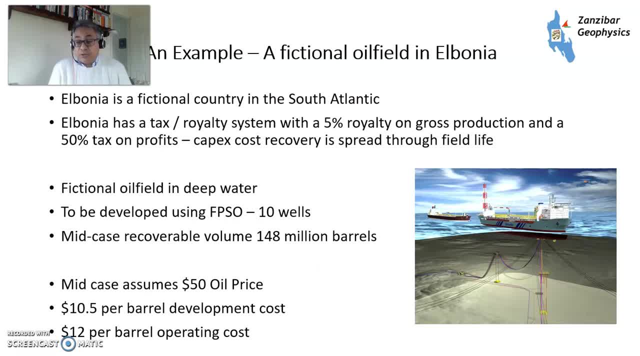 types of prices that are there. So we're going to look at a fictional oil field in the country of Elbonia, Fictional country. the South Atlantic has a tax royalty system: 5% royalty on gross production, 50% tax on profits. there's a 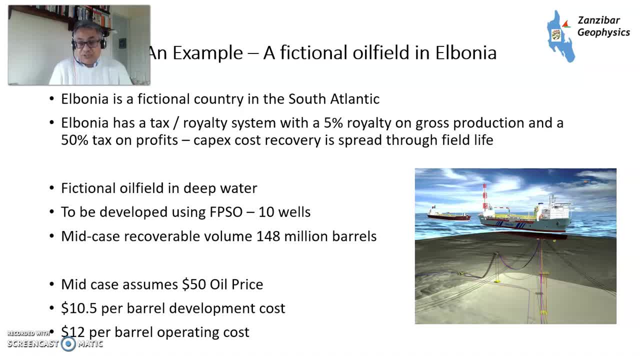 capex: cost recovery spread throughout field. life got a fictional oil field in deep water, FBSO, using a floating production system: 10 wells, 148 million barrels. it's an oil field. the gas will be re-injected mid-case. 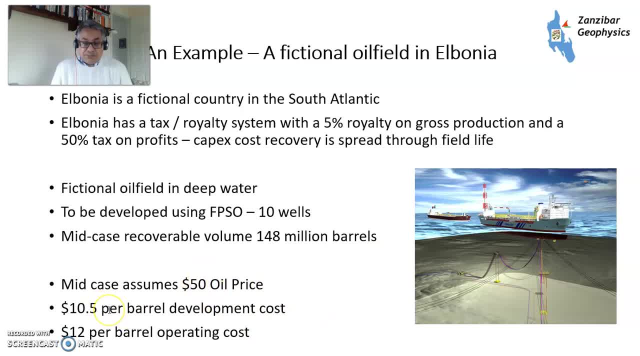 assumes $50 oil price, $10.5 development cost, $12 oil pricing cost, which are kind of roughly what you'd expect right now. I mean, obviously that would vary a little bit. we'll look at the sensitivities as well. So this is a 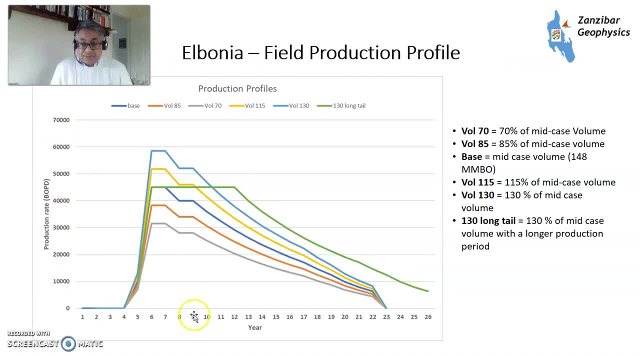 production profile. so that's a production rate in barrels of oil per day and these are the different cases. So volume: 70,, 70% of mid-case volume, 85,, 85% of mid-case volume. mid-case volume then 115,, 150%, 130% and 130% with a. 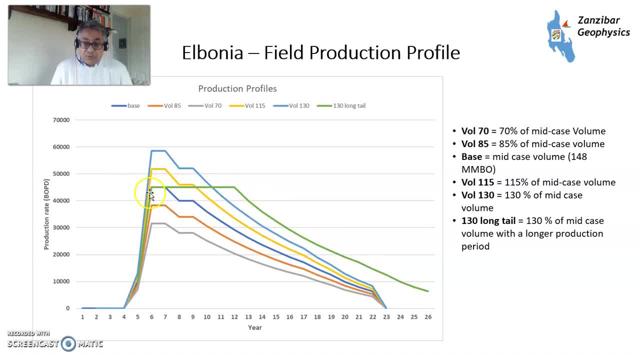 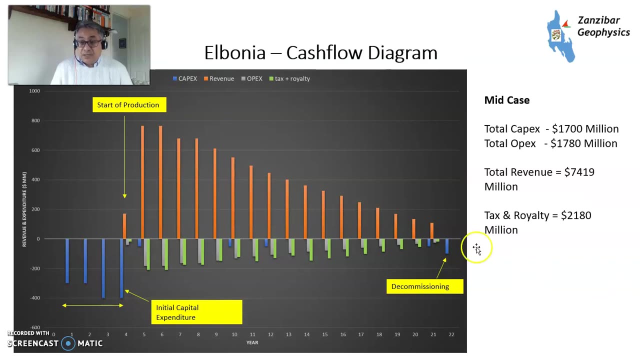 long tail where you cap a production rate. Now, obviously this would be the maximum production rate of the FBSO facility, and the long tail means that you can get away with building a small FBSO, but you just get a bit of production later. So again, we'll look at what these different things do. So 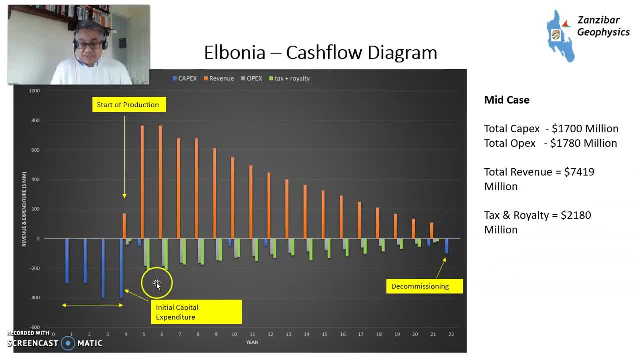 this is the cash flow diagram. So in blue is capex, in light blue is tax. then you have your revenue and then you have your OPEX and these are the little capex: infill, production infill, etc. and that's your decommissioning expenditure. so that's your start of. 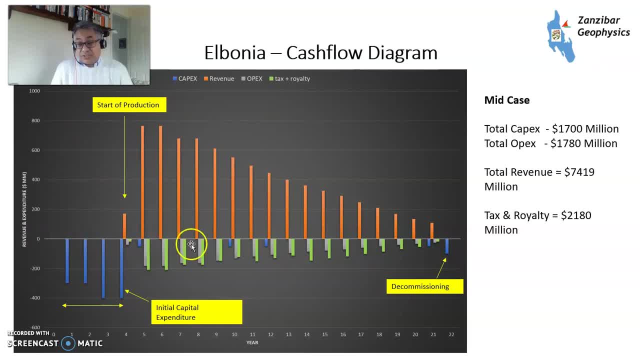 production. after about four years, which is roughly how long I feel like that would take to do So, you have 1.7 billion capex, 1.78 billion OPEX, 7.4 billion revenue and 2.1 billion in tax and royalty under this particular system that the 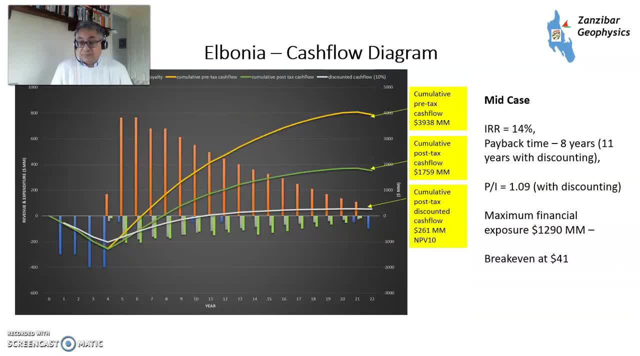 Olbonians have, and we'll come to how that varies in a minute. So this is your cash flow diagram. so that's your cumulative pre-tax cash flow. Yeah, that looks pretty healthy. Then this is after the government takes a share again. 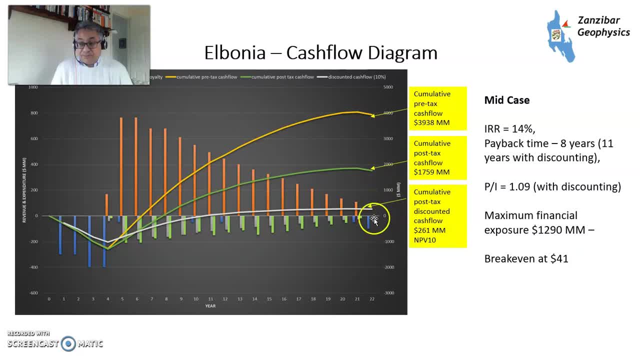 it's Olbonia's oil. therefore they take a tax and royalty share, and then this is after the cash flow discount, because what happens is that revenue at this part of the curve is discounted at 10% a year. So money coming in here is worth a lot less than money coming in here. Your. 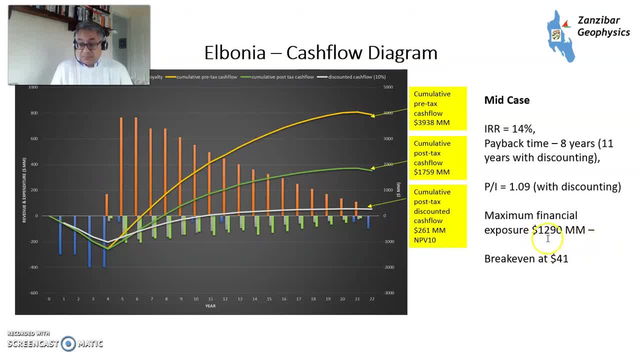 maximum financial exposure, 1.29 billion, and the break-even in this particular case is at $41.. So that's the different cash flow curves using cumulative cash flow. Okay, internal rate of 14%. that seems not too bad, Okay, but 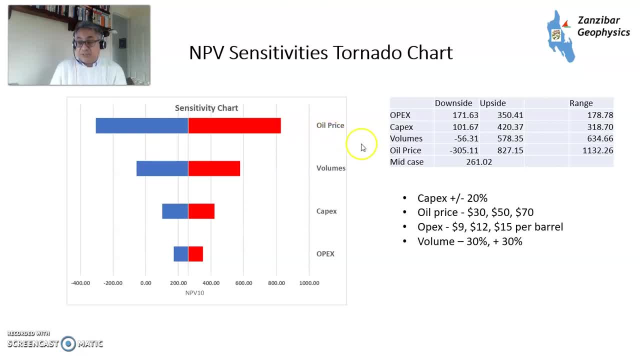 what if we got inputs wrong? So all the inputs are different. So we've got sensitivities here. we've got oil price, so we've got DEXA 30, 50 and 70,, OPEX at 9,, 12,, 15 a barrel and volume minus 30 plus 30.. So you can see. 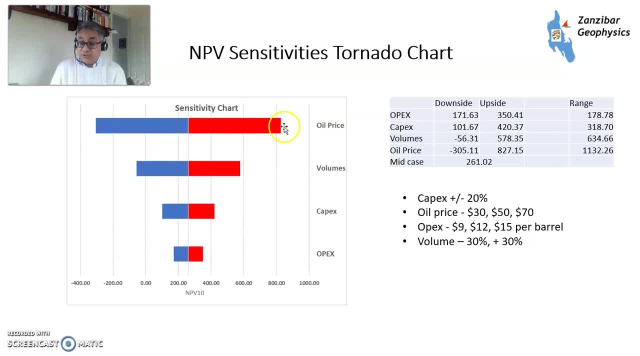 the big sensitivity here is actually the oil price. So if the oil price goes to $70, you make a heck of a lot more money with this particular tax system. Extra volumes give you a little bit more and volumes low. volumes are negative, so low. 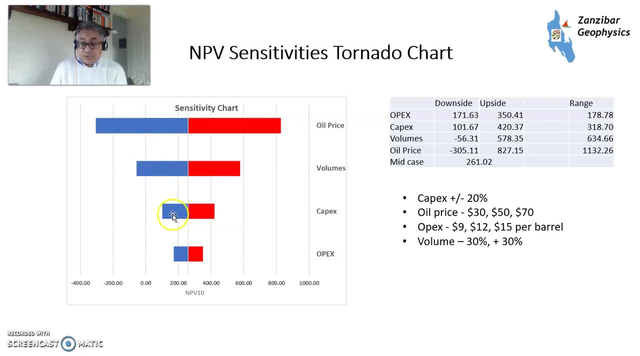 oil price, low volume are the things you worry about. Low capex: okay, it's quite a big discount, but not too bad. and then you've got OPEX, etc. And these are the different upsides and downsides. So this is a tornado chart that people use to explore. 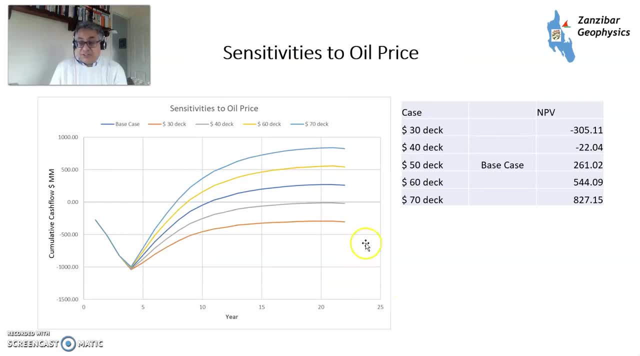 sensibilities. so these are different sensitivities to oil prices. So, using a $30 deck never going to fly Under these circumstances. Using a $40 deck. Well, we worked out: the break-even is actually at 41, so it's almost there. 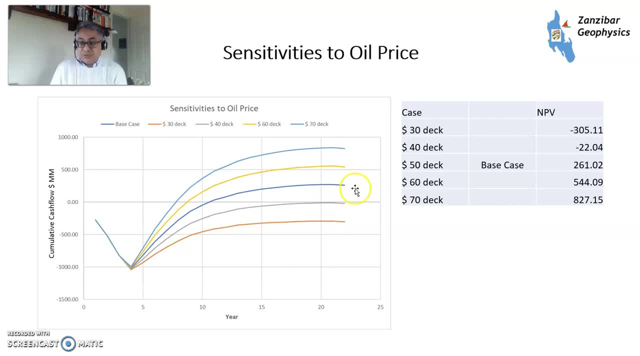 maybe you can shave off a bit of costs to try to get above the line, but it doesn't look too healthy. $50 looks pretty healthy. $60 looks very healthy. $70 looks very healthy indeed. anything obviously above that is dreamland. Well, it was when I originally did the work. 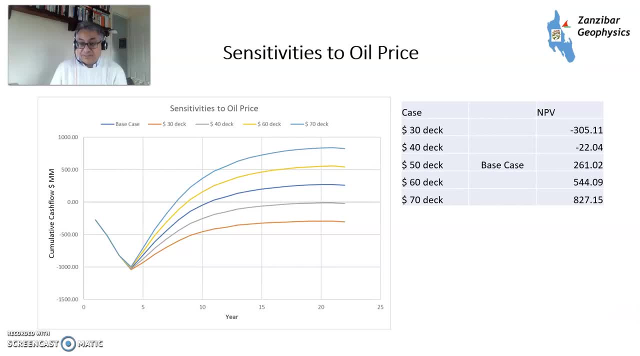 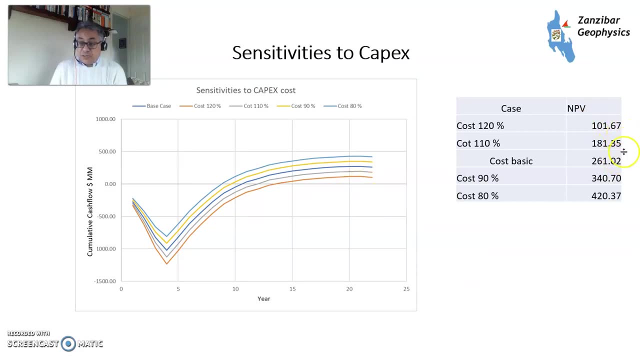 although current oil price is a little bit above that. but you can never rely on that. Sensitivity is on CapEx, so capital expenditure up front. So if you have a 20% overrun you lose quite a lot of value. If you have a 20% underrun, 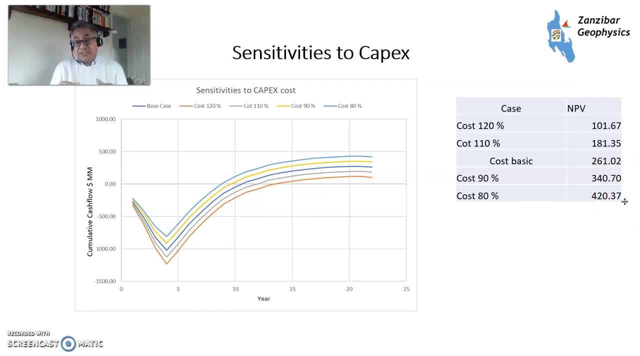 you gain quite a bit of value. So, looking and trying to optimize your CapEx to try to design things the right way and execute things the right way, which is actually the hardest part, you make a big deal. Sensitivity is the recoverable volume. So, again, if you get extra, 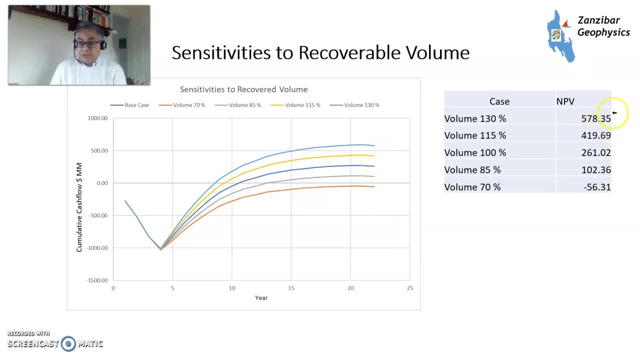 volume. if you have more than what you expected in terms of recovery, you get extra value. If you get less, it's 85%. you lose 15%. you're still okay. If you lose 30% of volume, less than what you think, not so good. So you want to make sure that you can strain that using 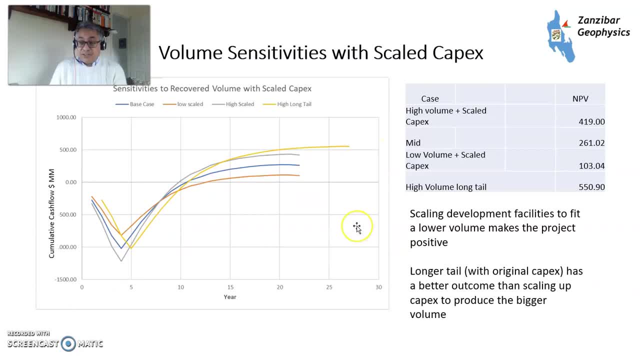 appropriate, appropriate Sensitivity is a scaled CapEx. So this is looking at well, what happens if we know that it's going to be the volume is going to be less or the volume is going to be more. So, for example, 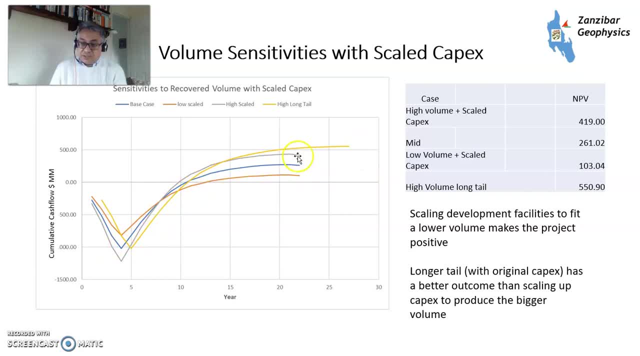 high volume with a scaled CapEx is looking pretty healthy, but the long tail where you use a mid case size FPSO just produced for a lot longer, gives you the best value of all, even though quite a lot of that is relatively late in life And if you have low volume but appropriately, scaled CapEx, you're going to lose a lot of value. So if you have a low volume but appropriately scaled CapEx, you're going to lose a lot of value. So if you have a low volume but appropriately scale CapEx, So if you know you're going to have a low volume, so you scale your facility. 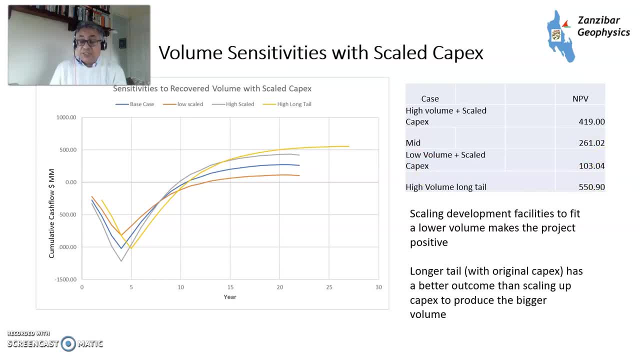 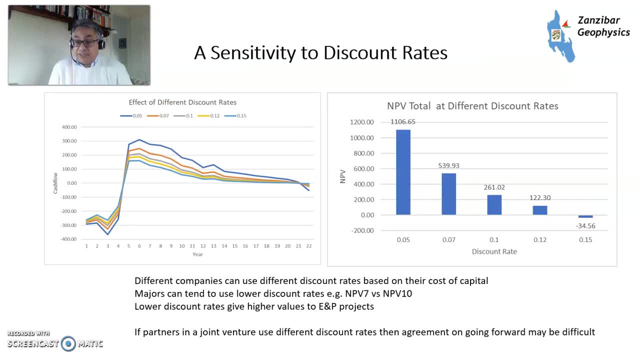 accordingly, you become positive. So again, appraisal works, knowing what you have works, trying to get that constraint as much as possible. Next one is sensitivity discount rates. Now, not everybody uses 10%: Some larger companies, particularly the majors, and maybe the state all. 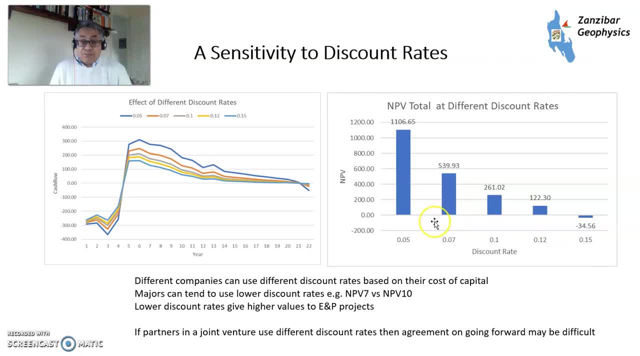 companies may use lower discount rates because they have bigger access to capital. For example, a major Asian national company may be funded by major national bank of that asian country. therefore the cost of capitals will be a lot less than this one independent. so you have a 10% discount rate. you get 261 7% discount rate: 539. 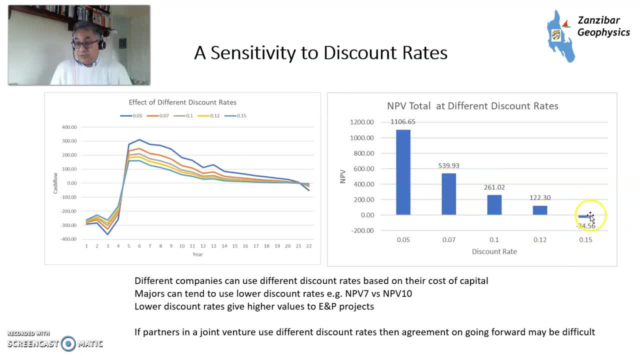 that looks a bit better, whereas if you go to 12 it's 122 and if you go to 15 it's negative. IRR was 14%. so if you're dealing with a small independent that has much more constraints in terms of capital than a larger company because they have to borrow money either through bonds. 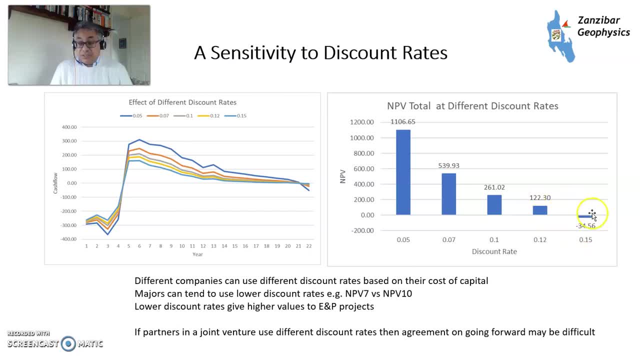 or bank loans, they have a problem. so maybe if you're a small independent, you might want to get out of this project by selling it to somebody to whom it is more value. but if you stay in there, you can have quite a big mismatch within a joint venture. and then sensitivity to tax changes. now 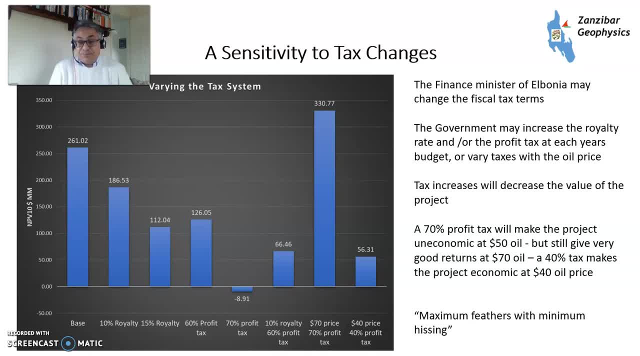 elbonia may think price has gone up. we want to take more tax. it's not just elbonia, britain's just done that as well within windfall tax and oil companies. so if you increase your royalties to 10, 15 percent you decrease the npv at um at your 50 price deck, 60 profit stacks or 15 royalty would. 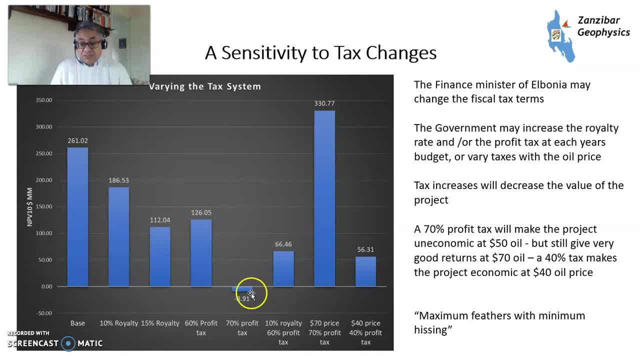 more than half the npv and if you take a 70 profit tax becomes negative at the 50 or price deck. if you take a 10 royalty, 60 profits tax, you know it's coming up to um, significantly less than uh than what we had before. you know less than a third. 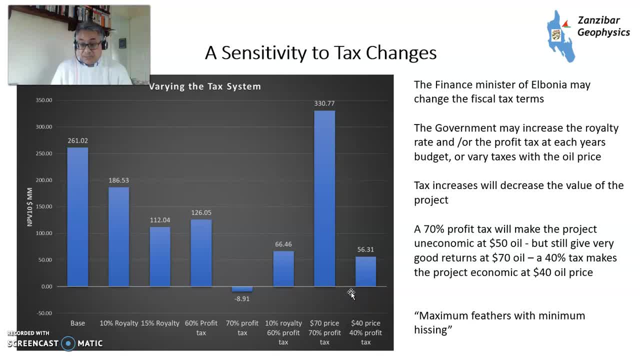 if you have a 70- 70 price deck. so all prices have gone up. the elbonian government has increased taxes. you get 330, still more than the original, but a lot less than 800. so elbonia takes a much fair, much larger share of the uh of the revenue as the 40 price deck but they may give 40 tax. that gets the project. 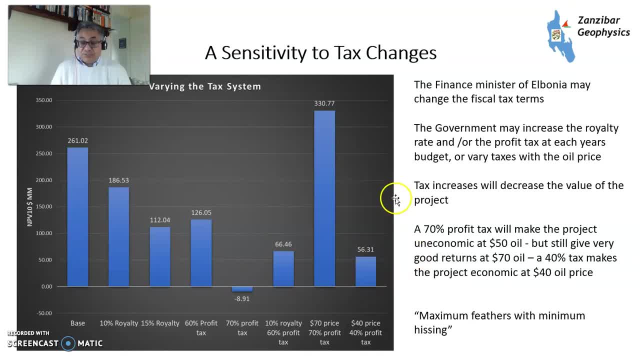 above the line. now, if the price goes up, the elbonia may increase the profits tax. now a french 17th century uh finance minister called colbert said you know, the art of taxation is maximum feathers, minimum hissing. maybe the elbonian finance minister is one of his disciples. 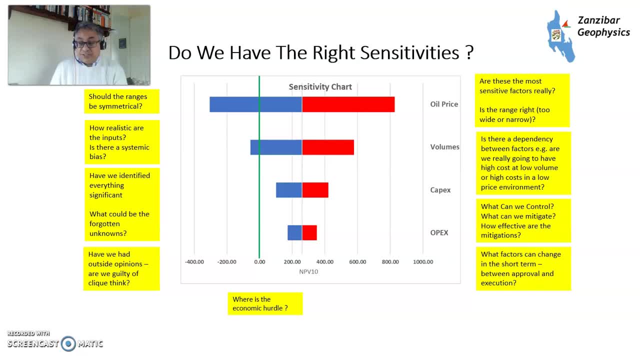 and the question that we need to ask as well is: do we have the right sensitivities? are these really the most sensitive factors? is the range right? you know people use a funnel, uh, you know, plus 20, minus 20 percent, etc. but is it too wide or too narrow? 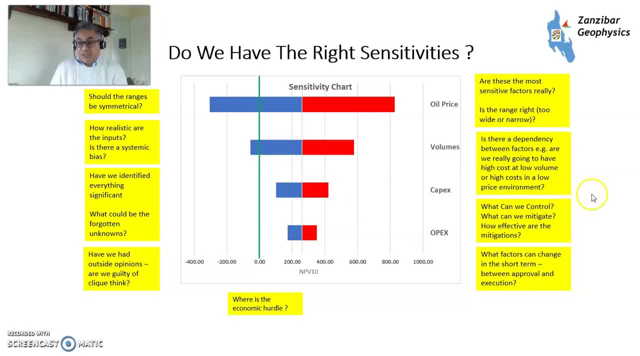 you know, is there a discrepancy. for example, you could have high cost or have high costs and low volume. you know high costs and a low price environment. we need to just check and double check what we do. what can we control, what can we medicate and how effective the 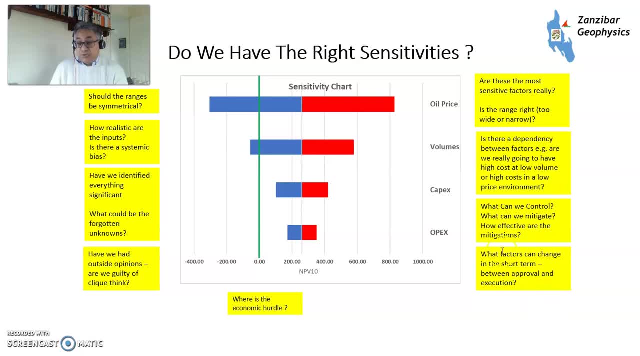 mitigations. you know discussions with the albonian government. what factors can we change in the short term between approval and execution? you know how can we do things better, how can we do things smarter? should the ranges be symmetrical? is there an asymmetric sensitivity that we need to look at? 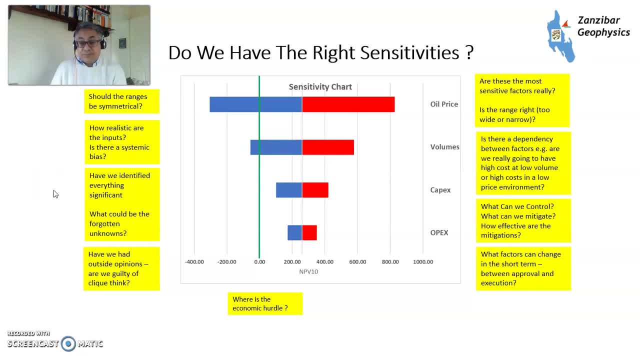 and how realistic are the inputs? is there systemic bias and have we identified everything significant? you know, what are the forgotten unknowns, what are the unknown unknowns that we can think of, and have we had any outside opinions? you know, are we guilty of clique think and where is the true economic hurdle? so that's something we need to think about.